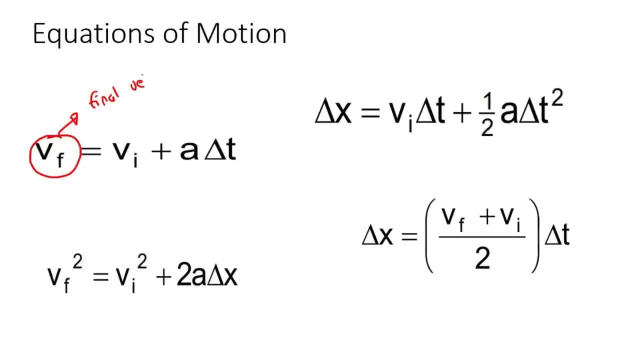 that stands for final velocity. Okay, whenever you see a VI, that stands for initial velocity, Whenever you see an X like that, it stands for displacement. Whenever you see an A, it stands for acceleration, And then whenever you see a T, it stands for time. Now there are going to be some type of questions. 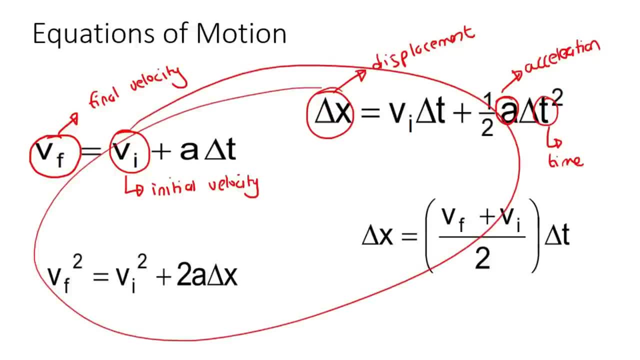 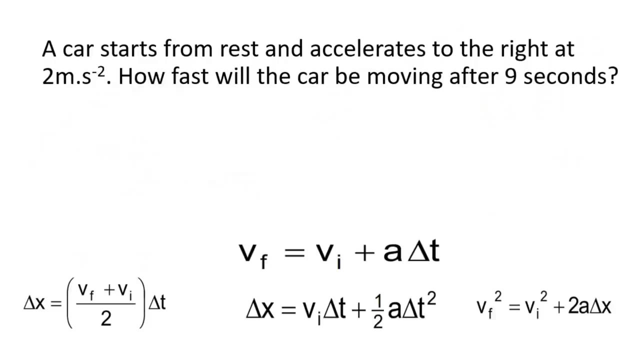 where more than one formula will work, Then you can use whichever one you like. You mustn't think that you only have to use the correct formula. Sometimes there's going to be more than one option available. Okay, but as we go through this lesson, I will make this very, very clear for you. So, 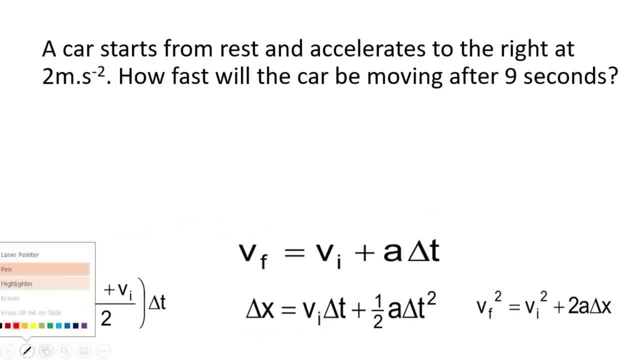 all I want you to do so. here we've got the four formulas again, and all I want you to do is read the question and then just go highlight whatever we have. So it says that a car starts from rest. Ah, if your car starts from rest, it means that your starting. 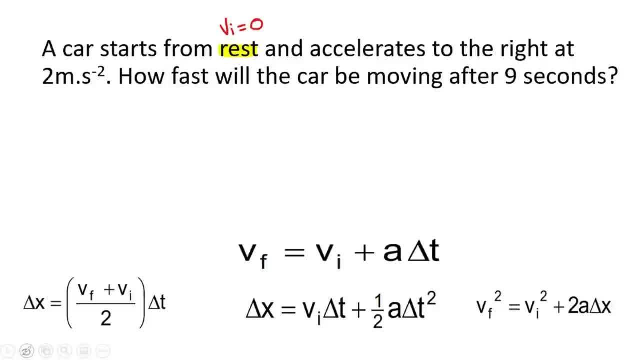 velocity, which is your initial velocity, is zero. Okay, so we have initial velocity. So I want you to go highlight initial velocity over here. Okay, so we'll highlight all of those. Then it says accelerate to the right at Ah. so we have initial velocity. So we have initial velocity. 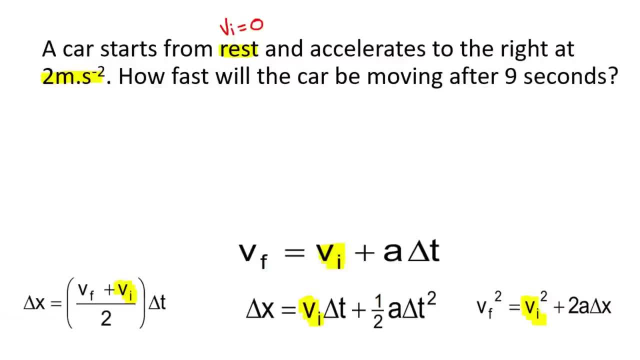 So they've given us acceleration. This is an acceleration, So let's go highlight all of the A's, A, A and A. Fantastic, How fast will the car be moving after Nine seconds? Ah, they gave us time, So go highlight all of the time. Okay, there and there. 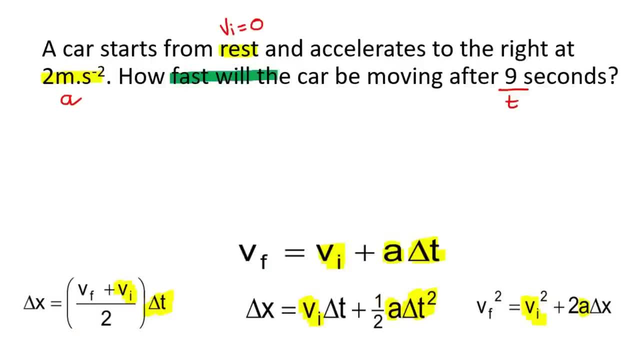 And then the question I want you to do in a different color: How fast will the car be moving? How fast? So they want to know what is VF, What is VF? So highlight that in a different color: VF. 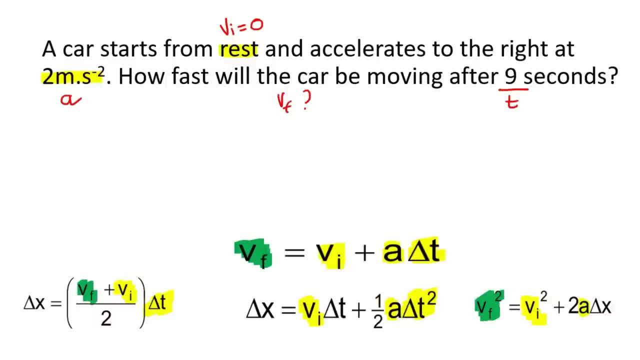 VF and VF. Okay, now I want you to look at these four formulas and I want you to see which formula has everything highlighted. Well, if you look at this one, VF is not highlighted, So we won't use that one. If you look at this formula: oh, that's not. 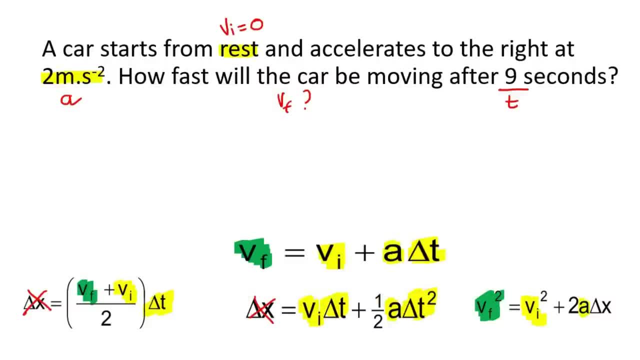 highlighted. I forgot to highlight the T there. Okay, I should have highlighted that T as well. But if you see, we can't use this formula because that's not highlighted. And then, if you look at this one, we can't use this formula because that's not highlighted. But if you look at this formula, 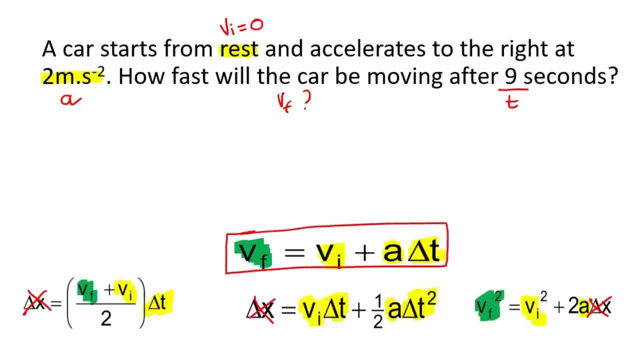 look at that. it has everything highlighted. So that is the one we're going to use. So in your test you would go write it down: VF is equal to VI plus A delta t. then choose a direction as positive. so they said that the car is accelerating to the. 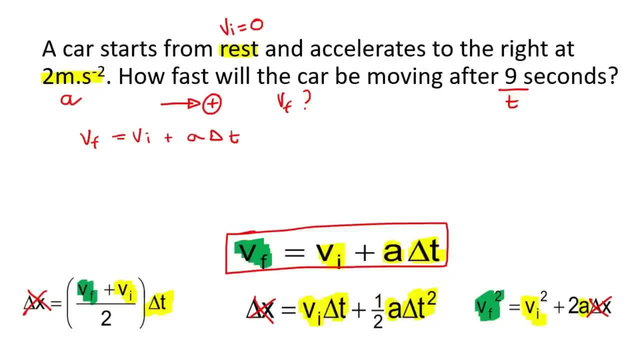 right. so i'm just going to choose right as positive. it will just make our life much easier. okay, so we don't know what the final velocity is. the initial velocity is zero, remember we said over there. then you're going to say plus a. now a is two, so you're just going to 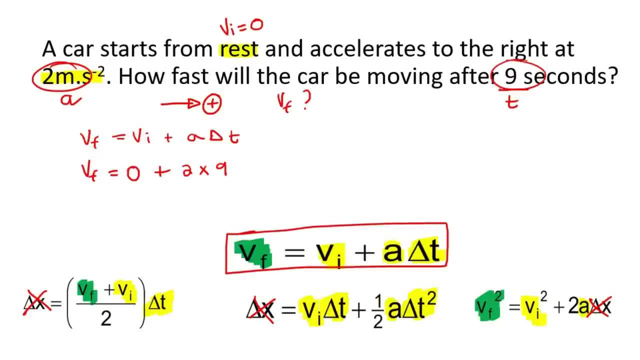 say two, and then the time is nine. so there, and if you had to go calculate that, you're going to end up with 18. now what is the units of velocity? it's meters per second. now, if you get a positive answer and you chose right as positive, then you can just say: to the right, okay, and so that is what we are. 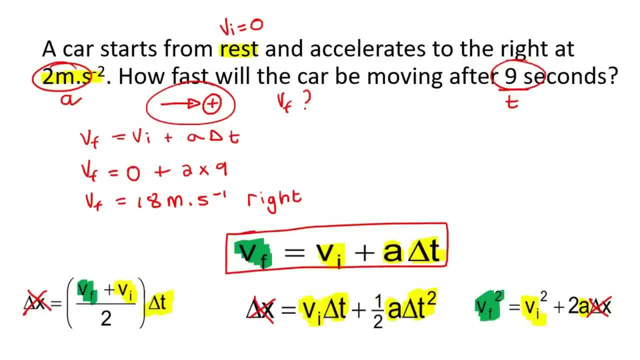 going to be doing for this lesson. you're going to be taking the question highlighting the different parts, choosing the right formula. sometimes in this lesson we're going to be doing questions where you're going to have to use more than one equation at a time. we're going to have to use two at a time. 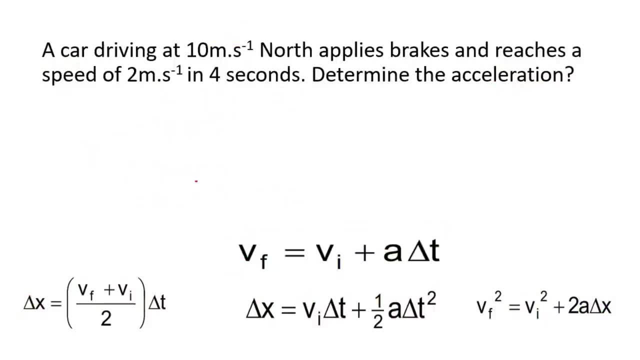 okay, but i'll show you that as we go along. okay, so here's our next one: a car driving at 10 meters per second. okay, so that would be the initial speed. so we'll say that that's the vi. so let's go highlight all of our vis, vi, vi, vi, because we don't know what formula we're going. 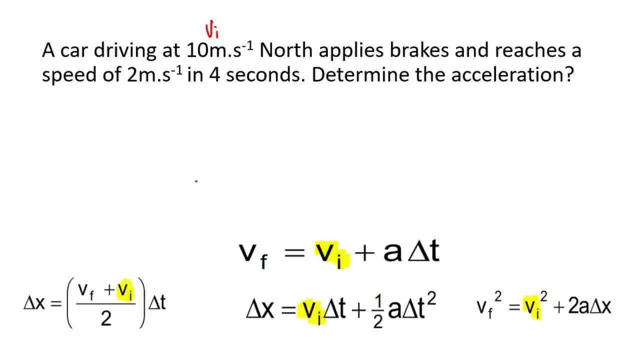 to use. okay. then it says it's driving north and it applies brakes and reaches a speed. okay, so this is the final speed. okay, so we go highlight all of the final speeds: final speed and final speed. okay, how long does it take? four seconds. they've given us time, so we go highlight all of the time: time time. 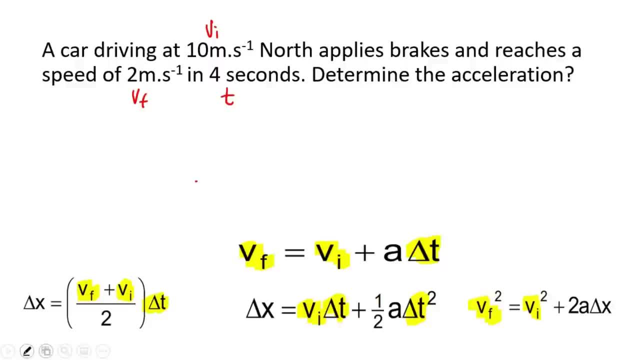 and that's it okay. then it says: determine the acceleration- okay. so that's what the question wants us to find. so highlight that one in a different color. so they want acceleration, acceleration, acceleration. now look for a formula that has everything highlighted. it all likes accelerating. so here it says: ave. 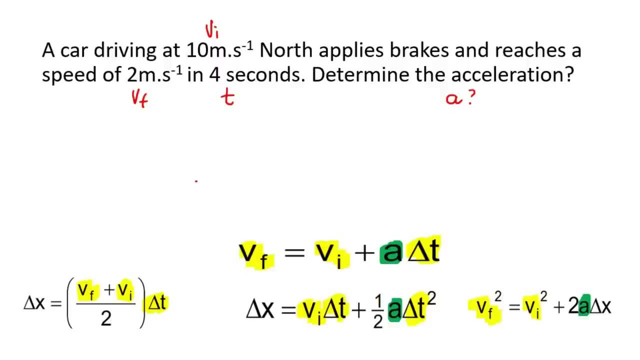 highlighted once again, it's going to be this one. okay, so what we'll do is we'll choose a direction, or let's first write down our formula: vf is equal to vi plus a delta t. choose a direction as positive. i'm going to just choose north as positive. um, north is positive, and so we can go. 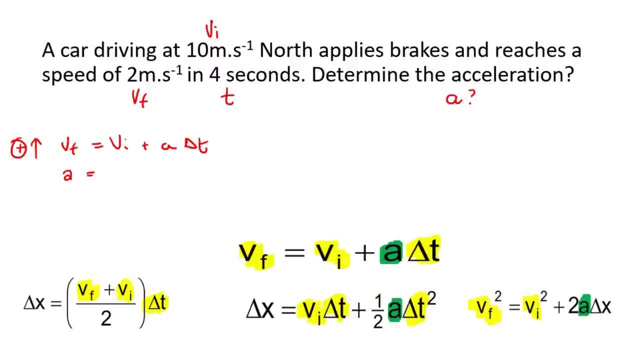 fill everything in now. so the final velocity was 2, the initial velocity was 10, the acceleration we don't know. and then the time is going to be 4 seconds. so we do that. now you need to solve an equation. so this is going to say: 2 is equal to 10 plus 4a, and then you need to get a by itself. 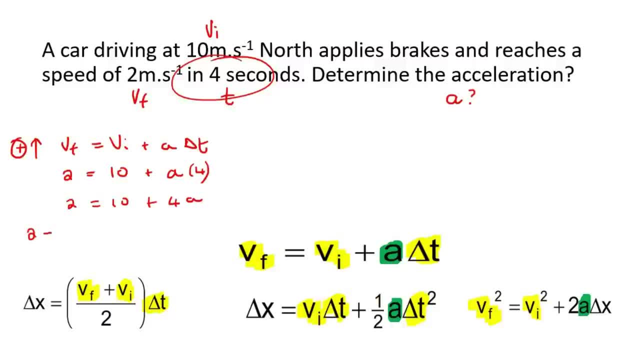 so i'll take the 10 to the left, for example. so you end up with: 2 minus 10 equals to 4a, and then 2 minus 10 is minus 8, like that. and then to get a by itself, we divide both sides by 4. 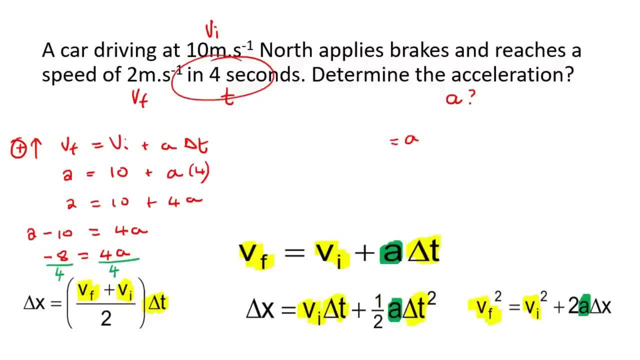 and so a would be negative two. so the way that you write that then is you change it to a positive two and then you put the correct units for acceleration. now we chose north as positive, but we got a negative answer. so we're going to say south two meters per second to the negative two. 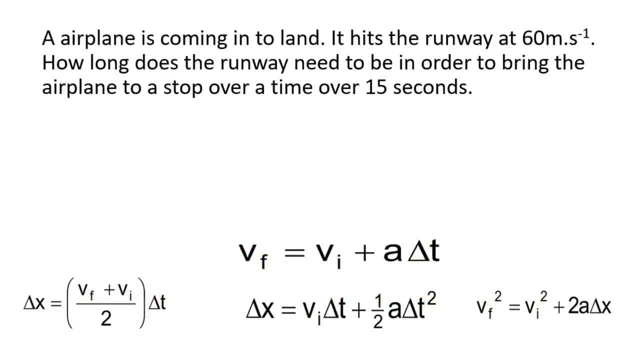 south. here's our next example. an airplane is coming into land. it hits the runway at 60 meters per second, so that's your initial velocity. so let's go. highlight initial, initial, initial and initial velocity. how long does the runway need to be in order to bring the airplane to a stop? 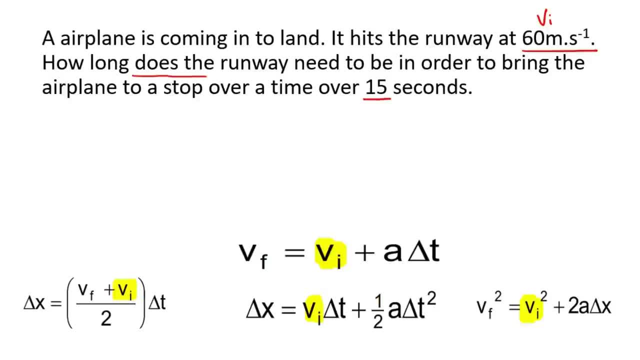 in 15 seconds, okay. so they want to know how long does the runway need to be, so if the airplane lands over here- a big airplane- and then it needs the long runway, and they want to know how long must that distance or that displacement be so that the 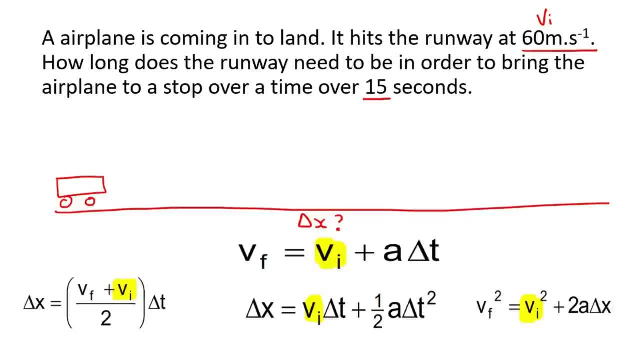 aeroplane will be in that distance so that después no necesita136.5 de' damas asset airplane can come to a stop. oh, we didn't even look at that. if an airplane comes to a stop, that's the final velocity. the final velocity is zero. if you stop, then you're not moving. 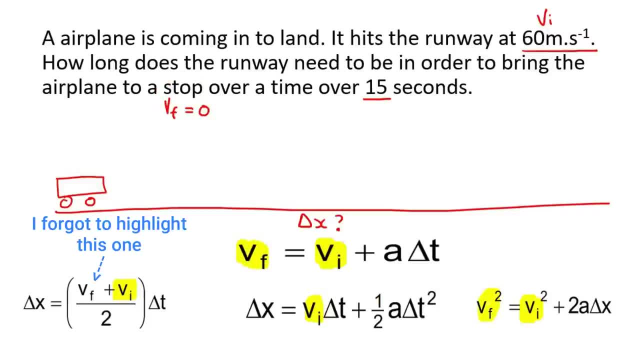 so they've given us the final velocities and they also gave us the time, 15 seconds, so we can fill in the time. and they would like us to calculate the, the displacement, which you can think of it as distance when we're moving in a straight line like this. now, if you look carefully, you'll see. 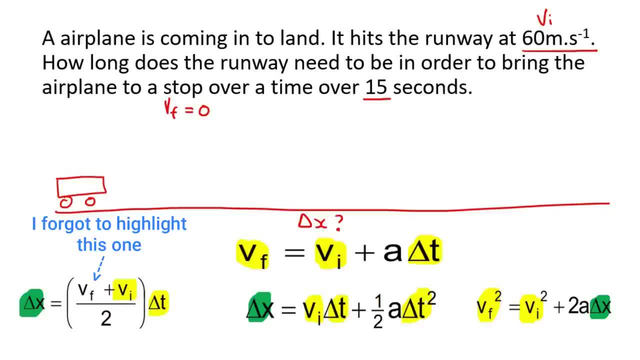 that there is no formula that has everything available to us. can you see that there is no formula that has everything highlighted. so what do we do? do we just abandon the question? no, i told you in the beginning of this lesson. sometimes we're going to need to use two formulas. 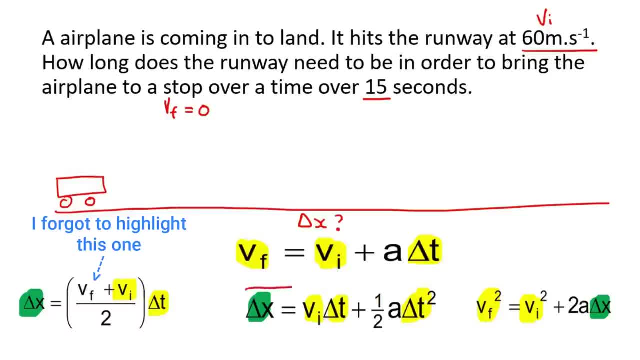 so, for example, this formula looks quite nice. the reason i say so is we're trying to find this one, and all that's missing is the time that we're going to use. missing is what's missing, guys. a so what we can then do is we can go up to this formula. 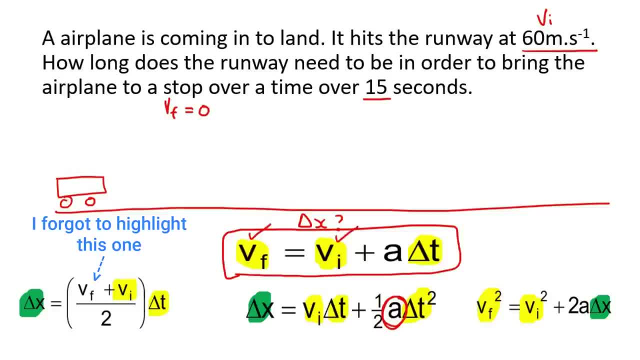 and because we know this and we know this and we know this, we can then use this equation first to find a, and once we find a, we can then come back down to this equation and just use that one over there. because you can't use this equation? because you don't know two things you don't know. 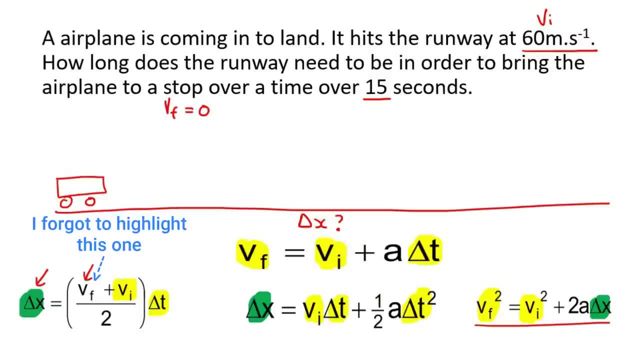 what that is. you don't know what that is. you can't use this equation because you don't know what. you don't know what that is and you also don't know what that is. so there's two things: you don't know and you can't use this equation because you can't. you don't know that and you don't know that. 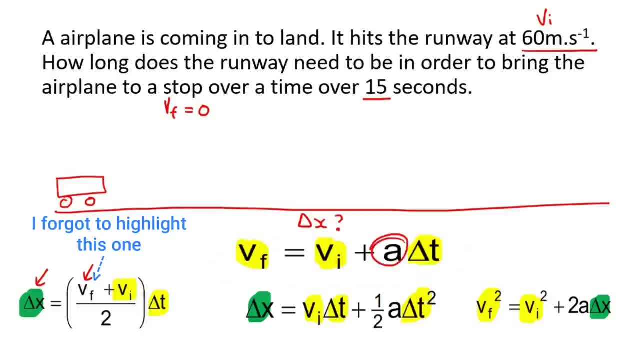 but we can use this equation because there's only one thing that we don't have, so we'll use this one and then, once we have a, we can plug it over there and then we can solve the rest of the question. so let's go: vf equals to vi plus a delta t. now they haven't given us any direction, that's okay. 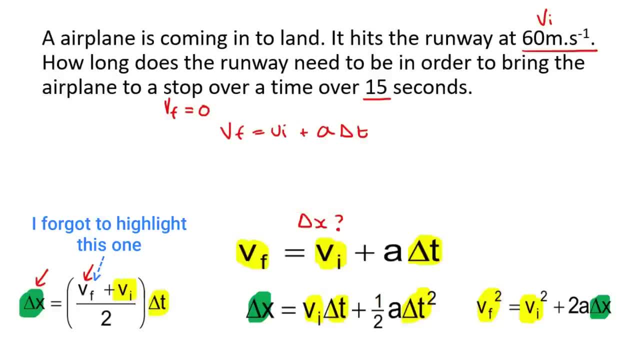 sometimes they don't. so what we'll do is we'll say 0 equals to 60 plus a, and then t is 15.. now if you had to say 0 is equal to 60 plus 15, 60 plus 15 a, then to get a by itself, you can take the 60 to the. other side, where it would be equal to 60 plus 15 a, and then you can take the 60 to the other side, where it would be equal to 60 plus 15 a, and then you can take the 60 to the other side, where it. 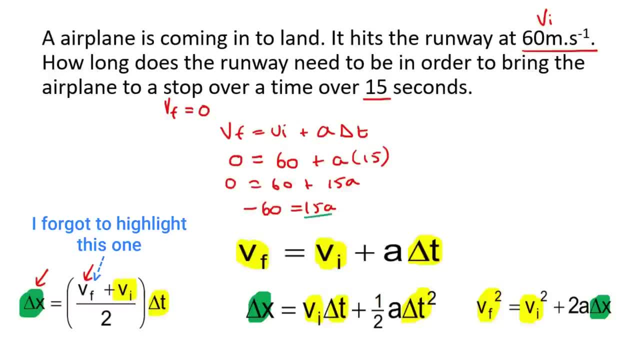 would be equal to 60 plus 15 a, and then you can take the 60 to the other side, where it would be will become a negative. now, to get a by itself, you divide both sides by 15 and you end up with- because this 15 then cancels and you end up with a equals to um negative four. why is the? 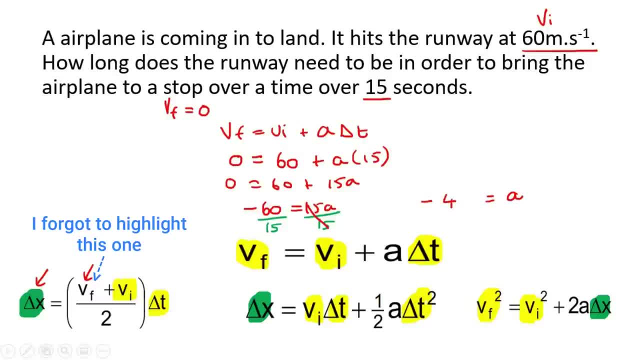 acceleration negative. well, think about it: when the airplane lands on the runway, we need the airplane to start slowing down, so we don't want it to be accelerating um, we don't want the. by having that negative acceleration, it means the acceleration is in the in the opposite direction to what we were moving, and so in this kind of scenario, it would mean that 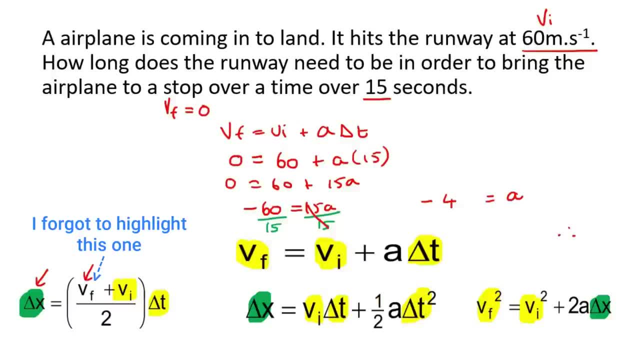 we are slowing down, and so we could say, therefore, acceleration is going to be equal to four meters per second. and then we can just say: here, in opposite direction, opposite direction of motion. now, here is the most important thing that i need you to understand when we go to. 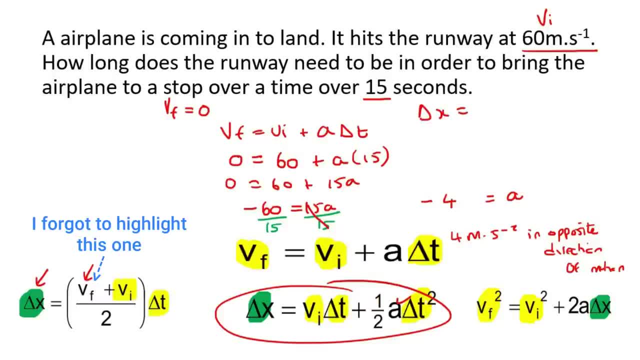 this next step over here. so we're going to go use that formula now. now remember that if the run, if the airplane, for example, is going in this direction over here, so it lands over here and then it's going in that direction. okay, now we need to find the distance of that um runway so we know that the 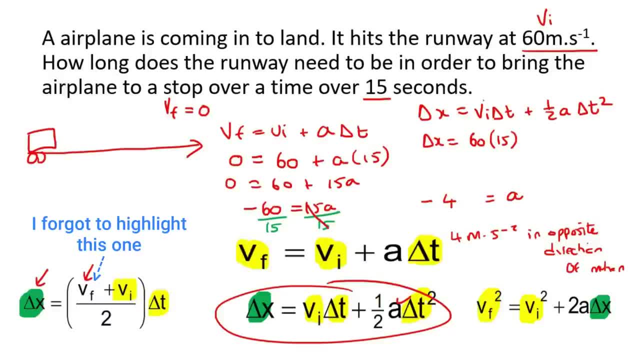 initial velocity was 60. we know that the time is 15, so we filled in that and we filled in that. then we say plus half now for your acceleration. you must put it as a negative because, remember, the object's going in this direction, so you're almost thinking of that as the positive direction. 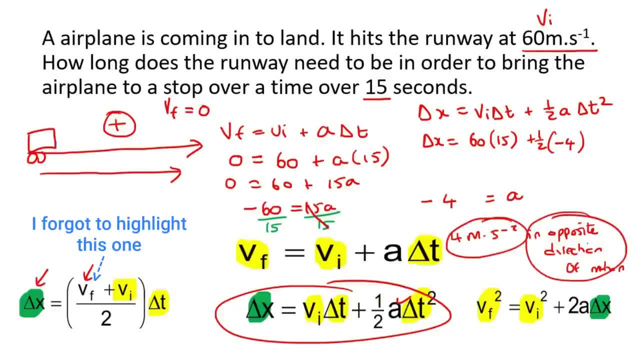 but the acceleration is four, but in the opposite direction. remember, we even got a negative four for the a value. so you're going to put a negative 4 over there and then, for the time, you're going to put 15 to the power of 2.. now, if you had to go calculate this, you end up with 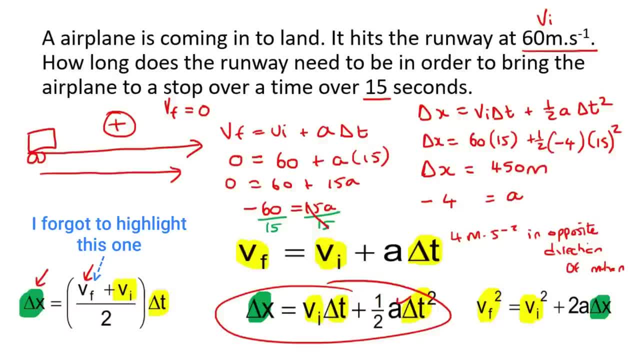 four, 450 meters, 450 meters. if you got a different answer, it's probably because you put a positive four over here, but that's not correct, because using a positive four over there, then you're saying that the airplane is becoming faster and faster and faster, and so you must make 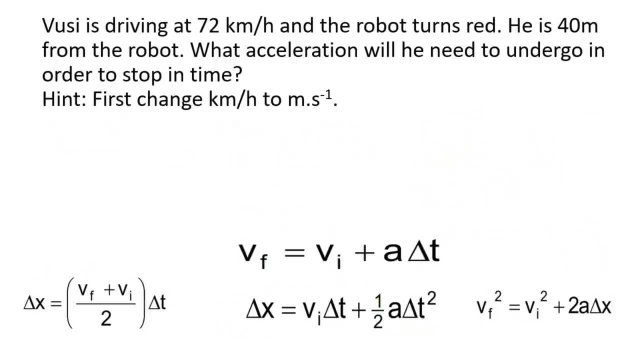 sure that this is the final answer that you got. here's our next one. this is a good question, because it gives us kilometers per hour and we need to learn how to change that into meters per second, because that's what the units that we work with. so vussy is busy driving at 72 kilometers per 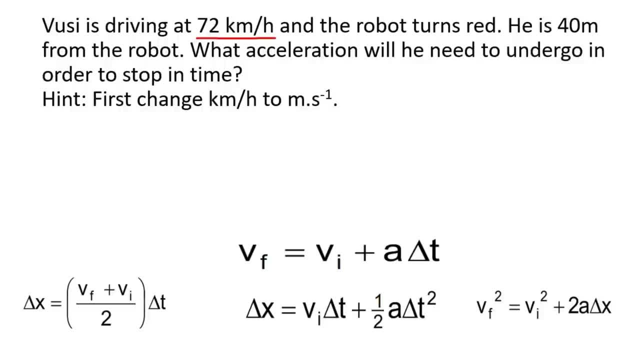 hour and the robot turns red. so he's busy driving and suddenly there's a robot in front of him that turns red. he is 40 meters from the robot. okay, what acceleration will he need in order to stop in time? okay, so we've got a person called vusi driving in a car and the car's. 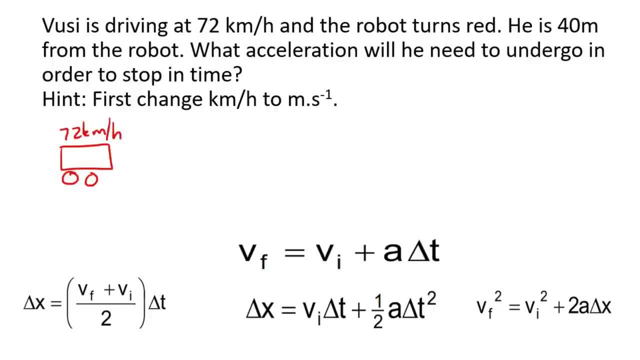 driving at 72 kilometers per hour. so we're gonna start with the performance we're gonna start with per hour. that is the initial velocity. obviously we need to first change it to meters per second, but we do have initial velocity so we can say we've got initial velocity, initial velocity. 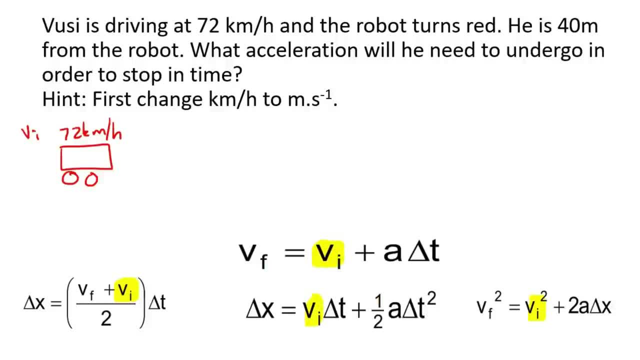 initial velocity. and initial velocity: he is 40 meters from the robot. so that is how far he is going to drive. that is how far he will go before he gets to the robot where he has to then stop. okay, so we have the displacement: it's 40. displacement and distance is very similar. 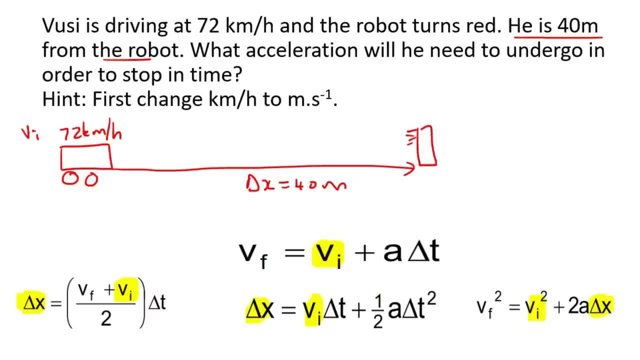 in this section. okay. and then it says: what acceleration will he need to undergo in order to stop? ah, if your car stops, then it means your final velocity is zero. so we have final velocity, we have that, so we can go fill that in. and then it says: 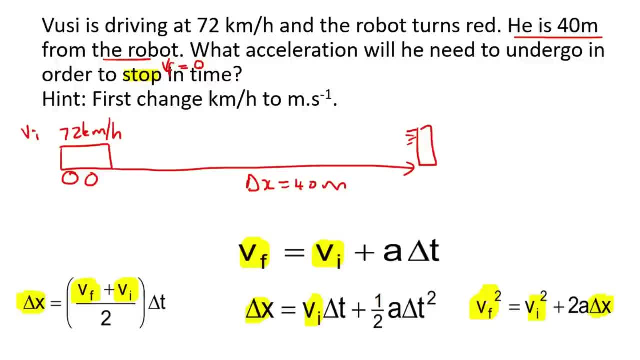 what acceleration does he need? so we are looking for acceleration. so what is acceleration? all right. so if you look at all the formulas, we're not going to use this one because we don't have that. we're not going to use this one because we don't have that. we're not going to use this one. 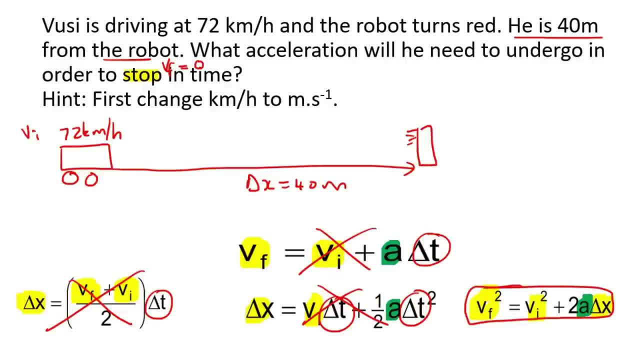 because we don't have the time, but we can use this one because everything is filled in. so we can just say: vf squared equals to vi squared plus 2a delta x. but now we need to first change kilometers per hour to meters per second. the way that you do that is you just do the following: you divide. 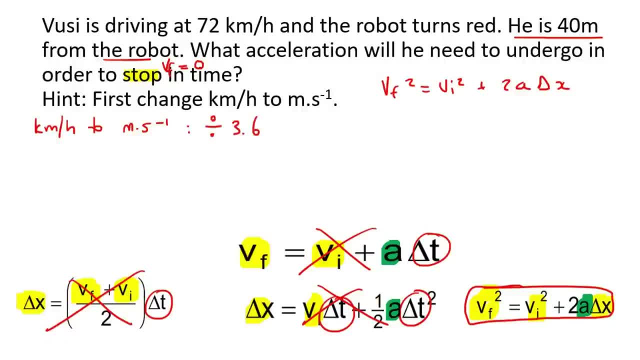 by 3.6. that is what you do. so you're going to take 72 kilometers per hour, you're going to divide it by 3.6 and that is going to give us 20, and that is what we will use. so the final velocity is zero. remember, we said that busi is going to stop. the initial velocity is 20. 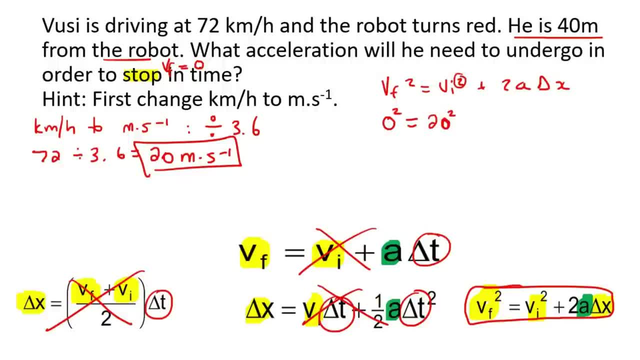 now remember, there is a little square over there. that's important. a lot of learners forget that. the a, we don't know. and then the displacement is 40. okay, now, what you do here is you just multiply everything together. so what is 2 multiplied by 40? well, that's going to give you 80, and then 20 to. 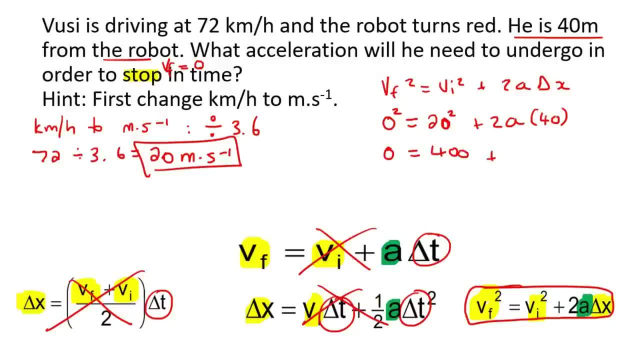 the power of 2, that's going to give you 400, and then this just gives you 80 a. now, to get the a by itself, you take the 400 to the left. now you divide both sides by 80 and divide by 80, and then you end up with a is equal to negative 5.. 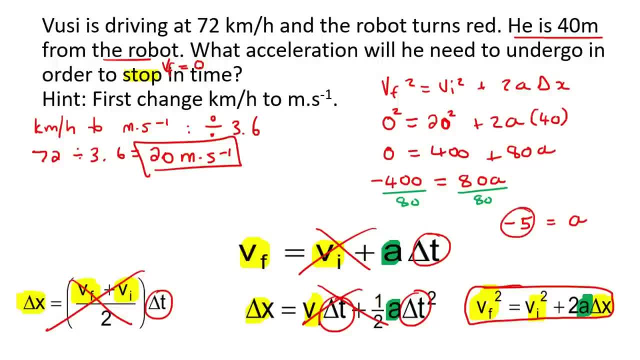 now the negative 5 for the acceleration. that should make sense. because you're slowing, because we're slowing down. the negative tells us that the acceleration is in the opposite direction to what we are moving. okay, so in these kinds of questions, a negative acceleration will tell us that we slowing down. but that's not always true, as I've 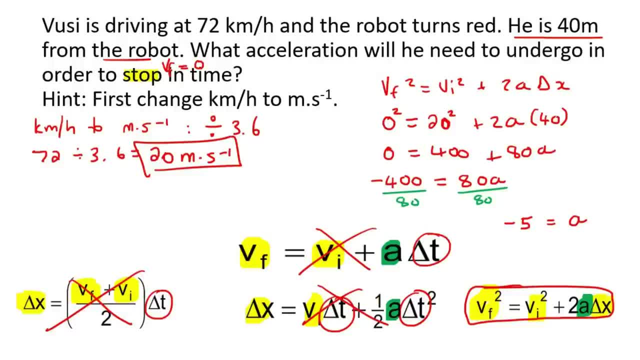 showed you in previous lessons. but in these equations of motion ones, then that's usually what's happening over there. so what we can then do is say a is equal to 5 meters per second to the negative 2, and then just say in the opposite, because they didn't tell us left or right is positive. we will just 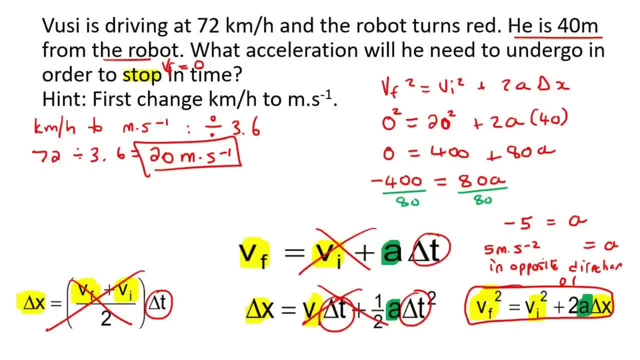 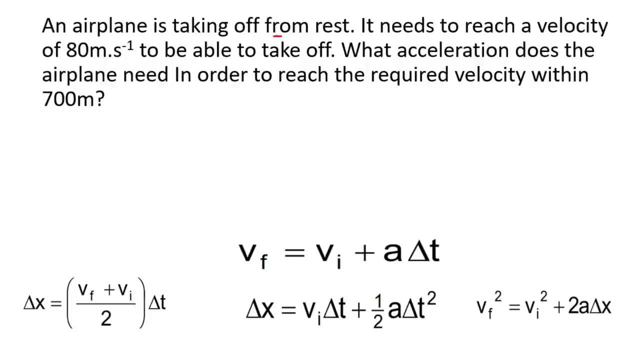 say in opposite direction of motion. Here's another one, an airplane as such has a continuous American here in the interviewing area of空 fry, the. the prelitль odin space strategy is" there's another one, and that is an airplane, is taking off from rest. ah, if you take off from rest, your initial velocity is zero. 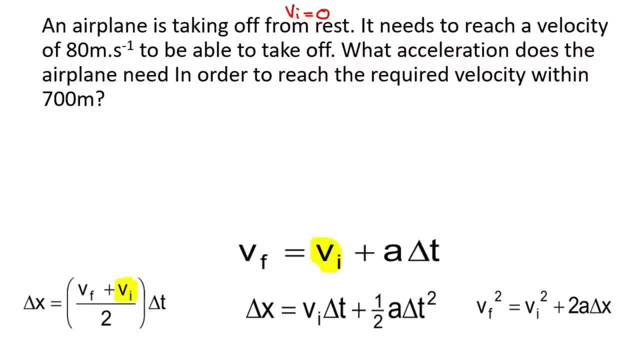 so we have an initial velocity. there we go, there we go and there we go. it needs to reach a velocity of 80. okay, so that's our final velocity that we need to reach. so we've got the final velocity. what acceleration does the airplane need in order to reach the velocity in 700 meters? okay, so that is your displacement. 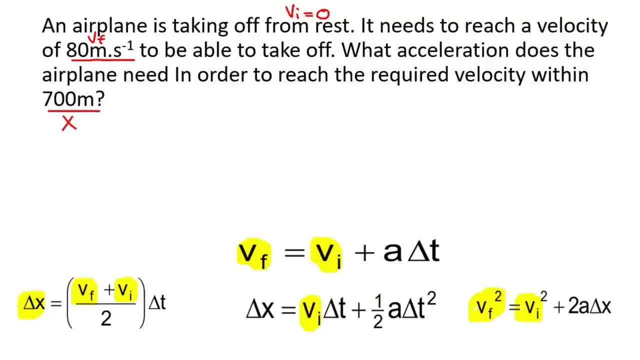 so we've got displacement, displacement and displacement, displacement. now they said: what acceleration? okay, so what is a? they want us to calculate a, so we can just go fill that in: a, a and a, and so if you look at the formulas, we can't use this one because there's um. no time, we can't. 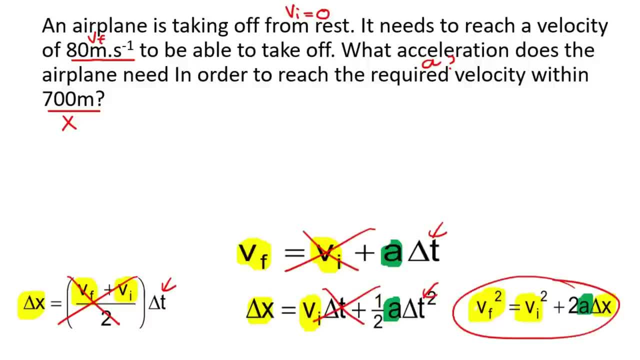 use this one because there's no time. we can't use this one because there's no time, but we can use this one. and so we can say: vf squared equals to v initial squared plus 2a, delta x, and the final velocity is 80, remember? the airplane is now taking off, so it starts at zero and then builds up at 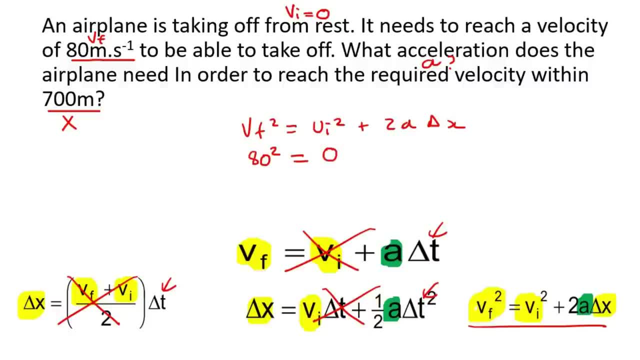 speed so that it can reach 80, then the initial velocity was zero, the acceleration we don't know, and then the displacement is 700. so if you type this on your calculator, it'll give you 6400. okay, then zero to the power of two is just zero, and then this becomes two multiplied. 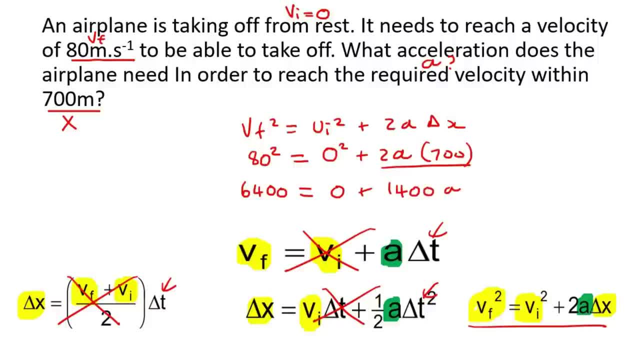 by four, and then the initial velocity is going to be zero, and then the displacement is going to zero, and then the initial velocity is going to be zero, and then the initial velocity is going to be two by 700, which is 1400, a. okay, now zero just doesn't really do anything. so we just do that. 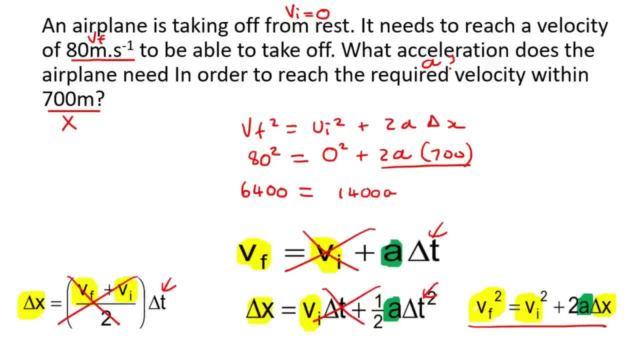 we can actually just write it like that now: to get a by itself, we divide both sides by 1400, and so on the left we end up with 4.57, and then on the right, these cancel, so you just get a. so that means a is going to be 4.57 meters per second, and then we can just say: um. in original: 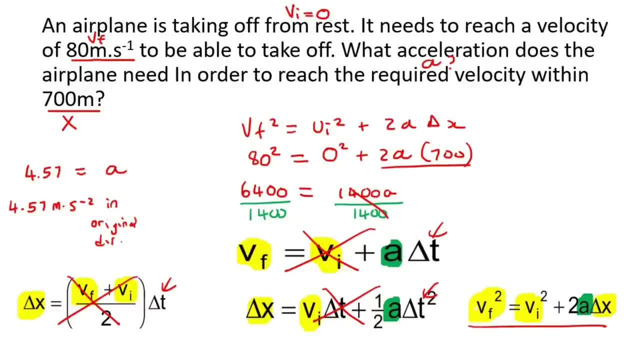 direction because we got a positive answer. they didn't give us what positive and negative is, so we can just say: in original direction okay, and so it makes sense that the airplane has a positive acceleration. in this scenario it's going with um the original direction because the airplane is. 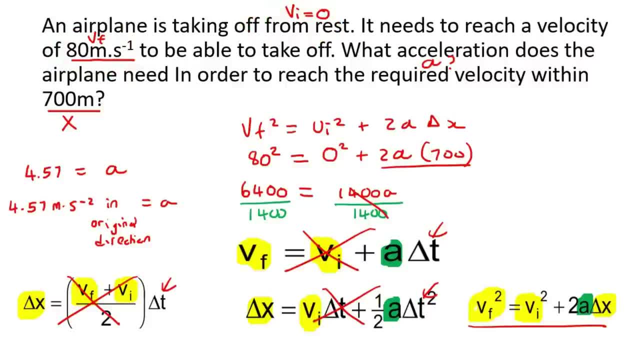 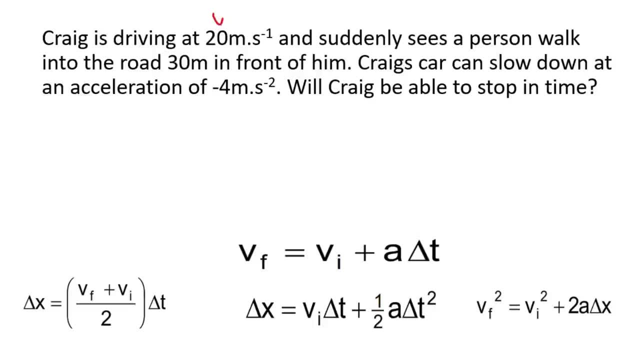 going from zero up to 80 meters per second. here's our last one. craig is busy driving at 20 meters per second. okay, so that's the initial velocity, initial velocity. so if we go, highlight that initial, initial, initial and initial and suddenly sees a person walk into the road 30 meters in front of 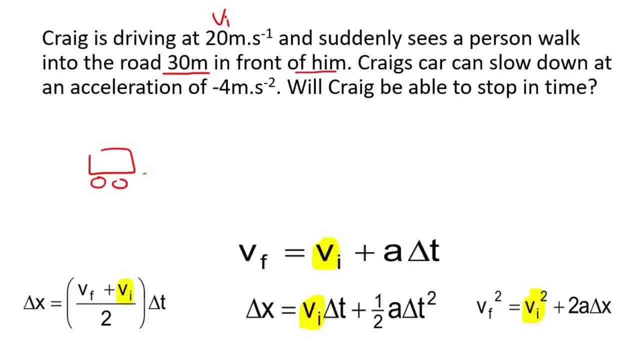 him? okay. so craig is busy driving his car over here and then, 30 meters in front of him, someone walks into the road. okay, so we have the and it says craig's car can slow down at an acceleration of that. will craig be able to stop in time? okay, so let's pretend that craig will. 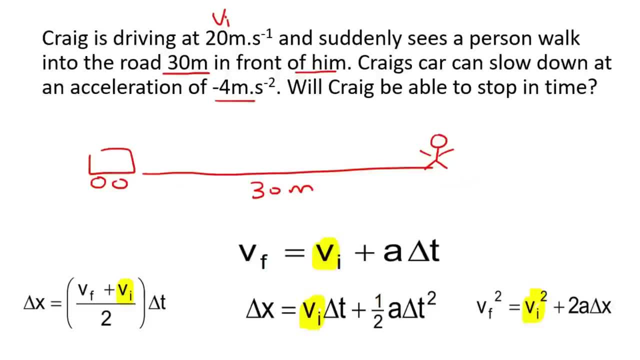 stop in time so that the total displacement is going to be 30. so we'll take that as 30. so we have that. they then say: craig's car can slow down at an acceleration of negative four. the negative is just because we are going to be. 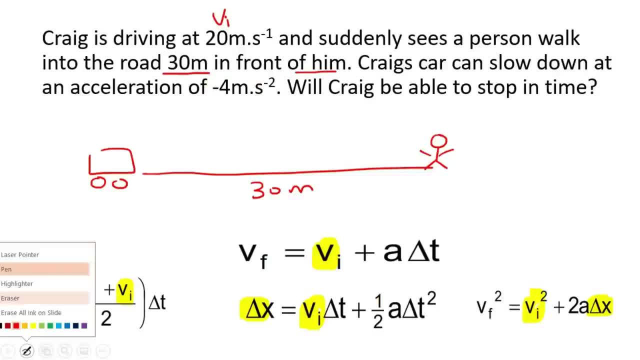 slowing down in this type of scenario. so we have the acceleration, we can go fill that in. will craig be able to stop in time now? i'm going to show you a little trick in this question. okay, this one's a little bit of a sneaky. 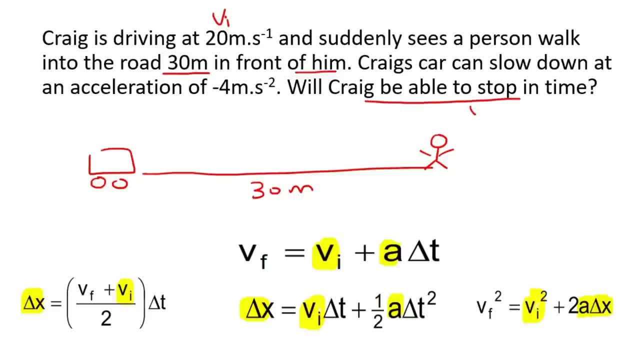 one. we know that craig needs to stop, so that means the final velocity will be zero, but we don't know if craig will stop in time. we don't know if craig's going to stop in time. we don't know if craig's going to be able to stop in time, so we don't know. so what we can do is we can then go. 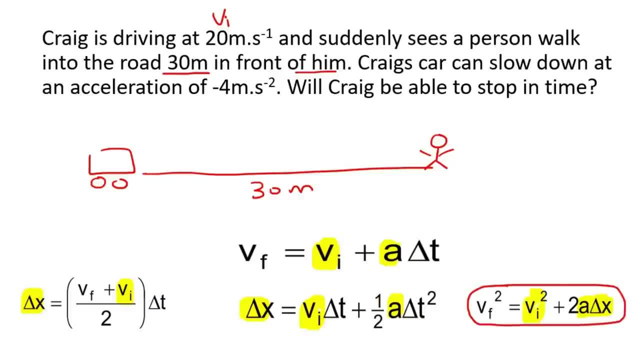 we can then actually use this formula over here and what we can do is calculate the final velocity, and we want to make sure that craig's car will be able to reach zero. let's see. let's see what craig's final velocity is going to be. 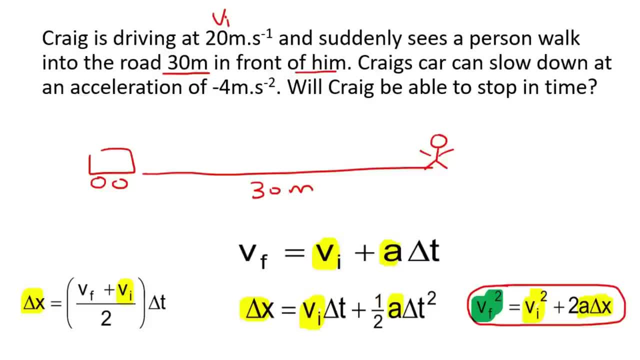 so we could say: vf squared equals to v initial squared plus 2a delta x. now we can say that we don't know what the final velocity is. we hope it's going to be zero so that craig can stop before he hits this person. but let's see. so the initial velocity is 20 and there's a to the power of two. now the 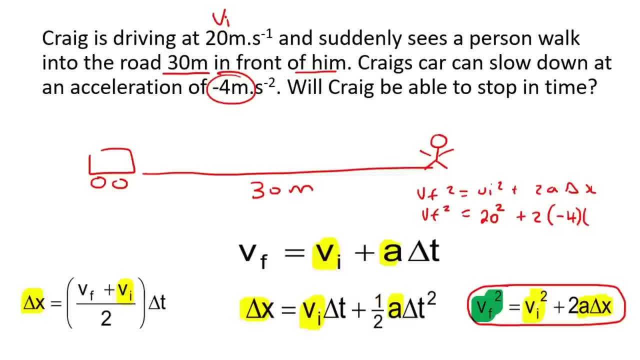 acceleration is a negative number, so remember that. and then the displacement is 30. okay, so if you had to go work this out, you're going to end up with 400 minus that's 240 over there. so then vf squared is going to be 160 now to get the. so if you've got vf, 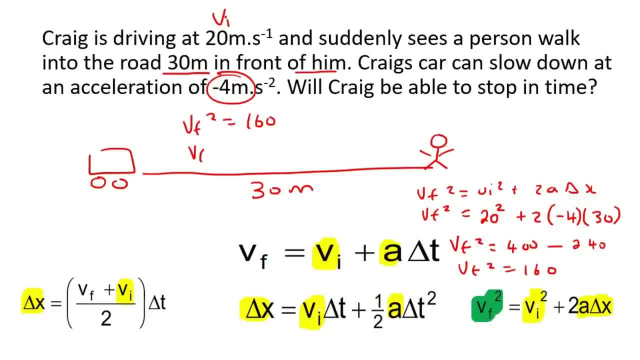 squared equals to 160, then to get the final velocity you have to take a square root, and if you take the square root of 160, you end up with 12.64- sorry, 12.65- meters per second. so that's what that means. is that, unfortunately, sorry guys? this is a bit of a graphic question, but this person's 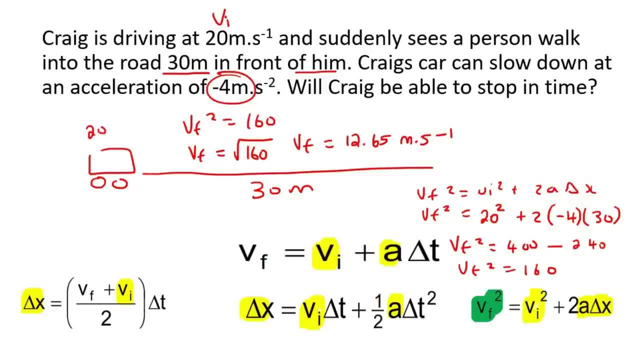 going to be bumped over because craig is driving at 20 meters per second. by the time he covers 30 meters. he's only driving 12.65 meters per second, so his car has not come to a stop. so he is actually going to collide all into that person. so will craig be able to stop in time? no hope that makes. 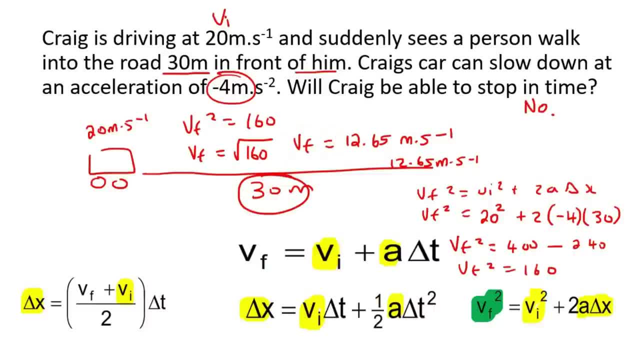 sense. so, um, what we did is we went in, calculated his final velocity and we realized that it's not going to be zero, it's going to be 12.65, so his vehicle is not going to stop in time.